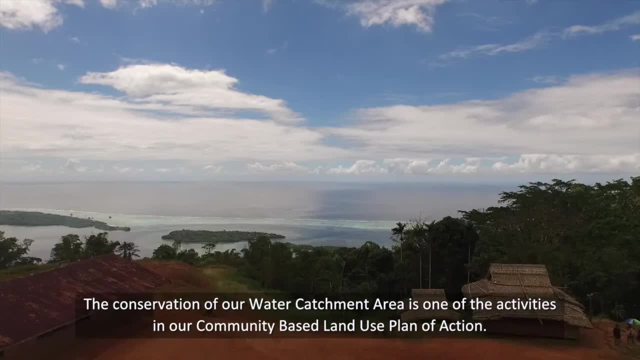 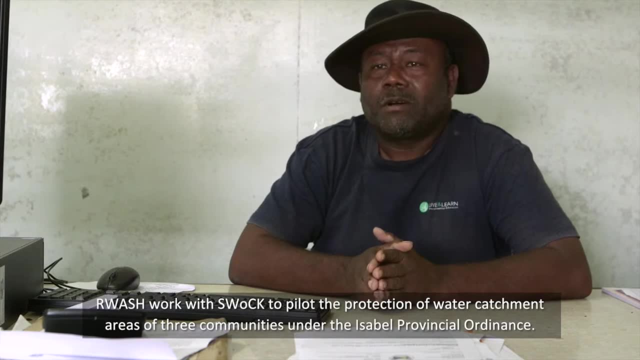 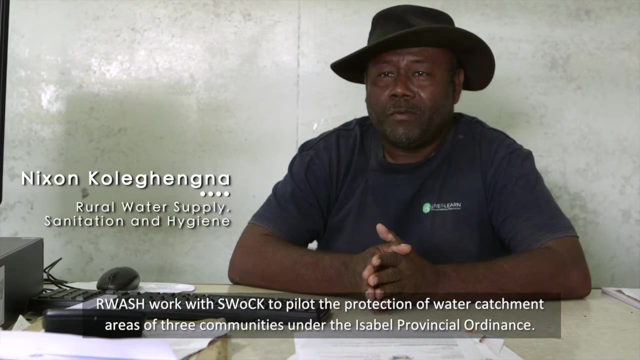 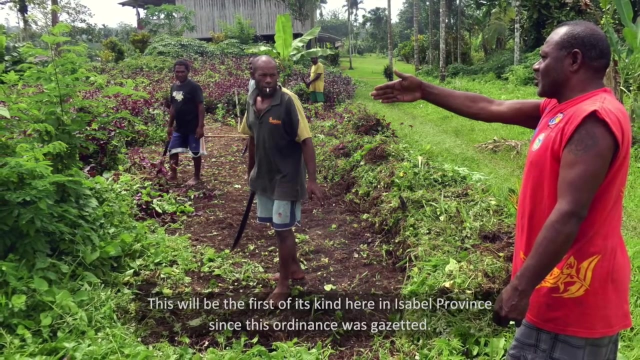 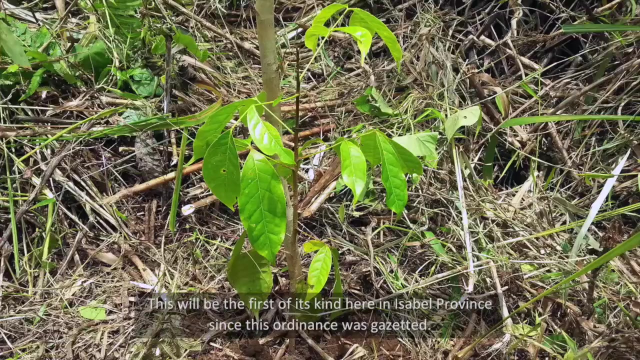 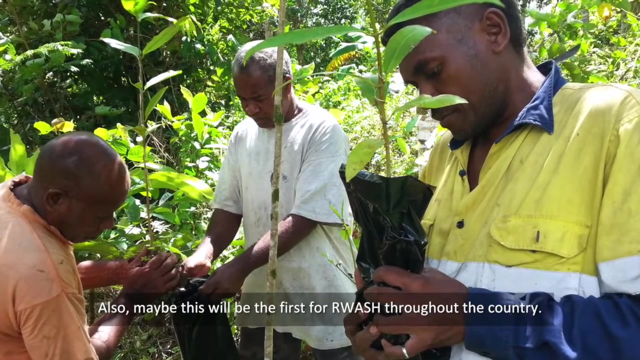 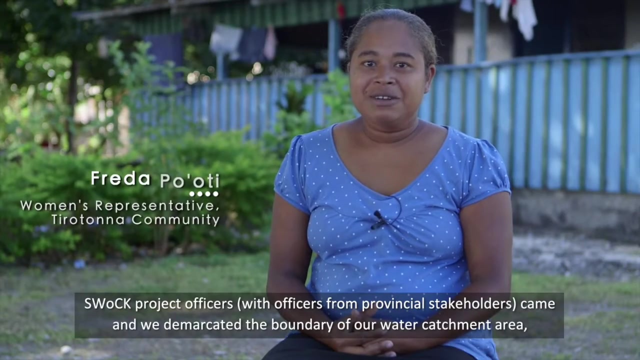 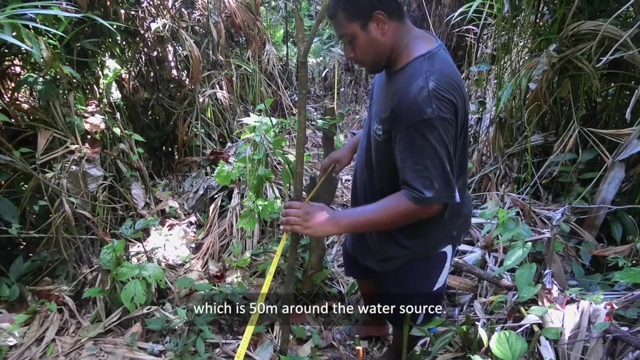 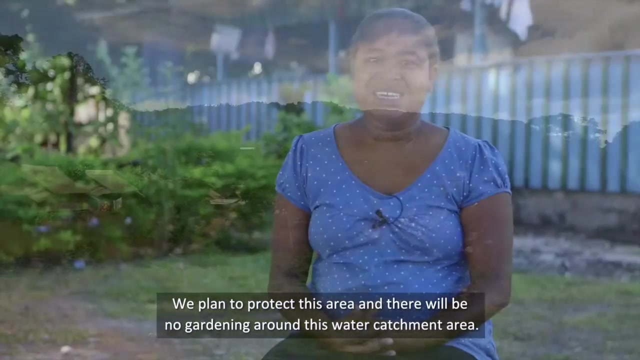 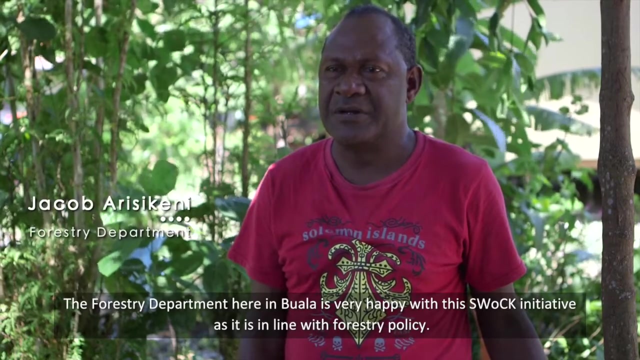 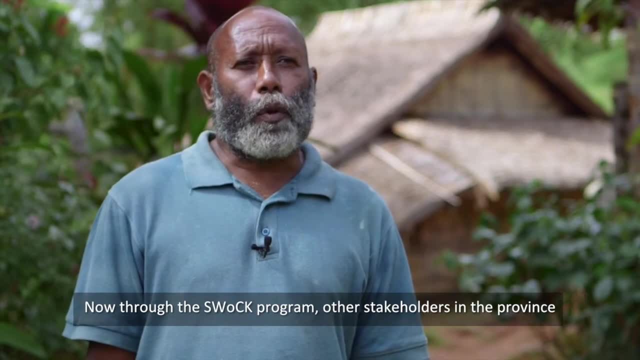 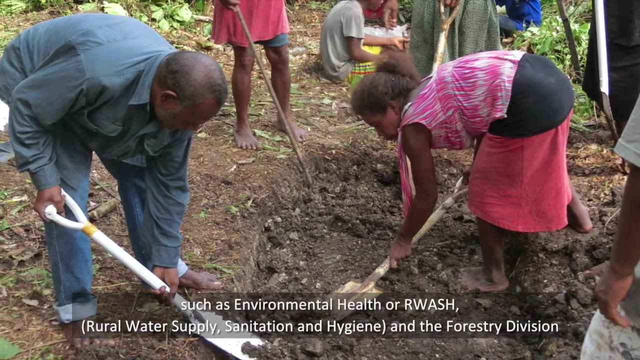 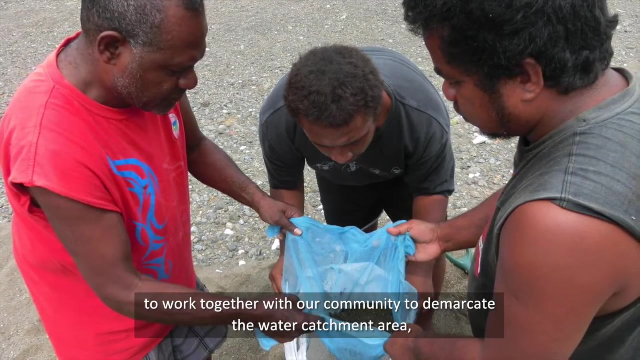 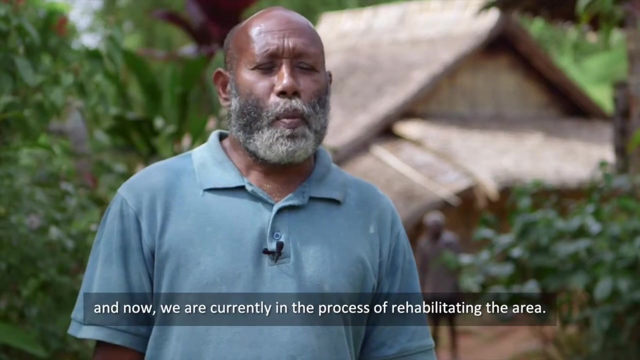 So now, through the SHOC program, he is asking other stakeholders of the province, like Health, Environment or ARWAS and the Forestry Division, to come up and help the Mifala community to demarcate the area, And now it's on the process of rehabilitating the area. 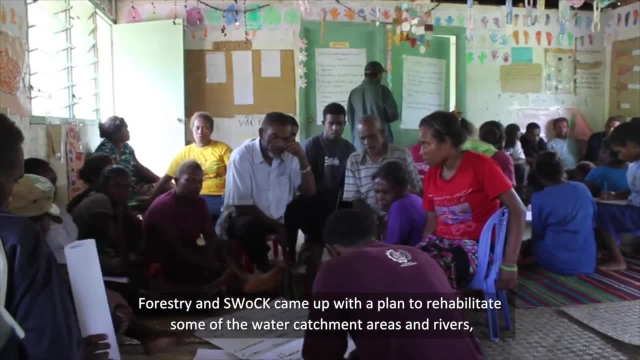 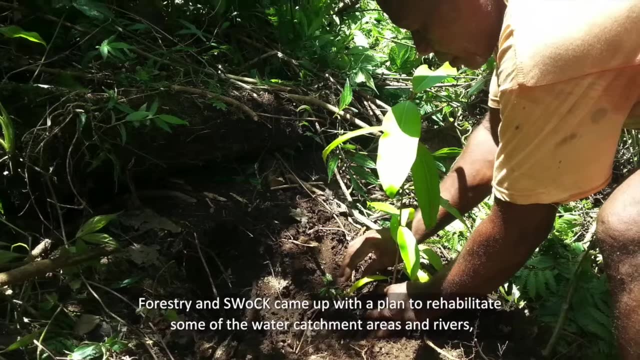 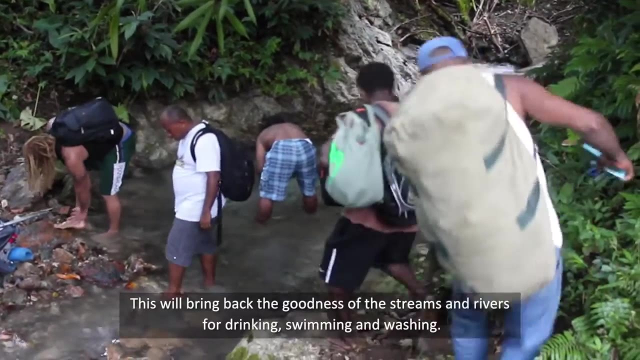 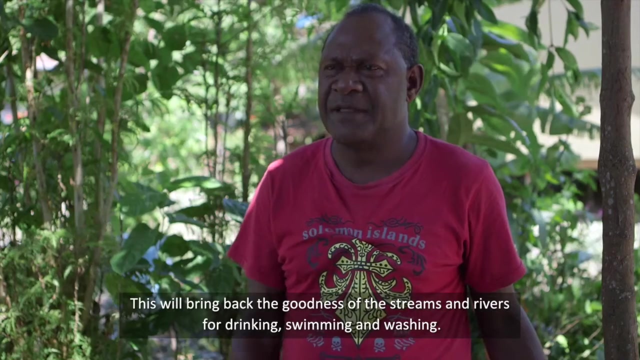 The idea of where Mifala came up with, especially forestry and SHOC, is for rehabilitating the water catchment areas and rivers, And the community has a lot of this, So now we are bringing it back, getting the streams, rivers for drinking and for swimming and for what's what. 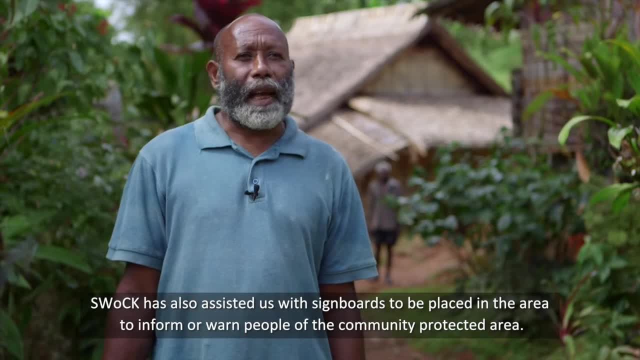 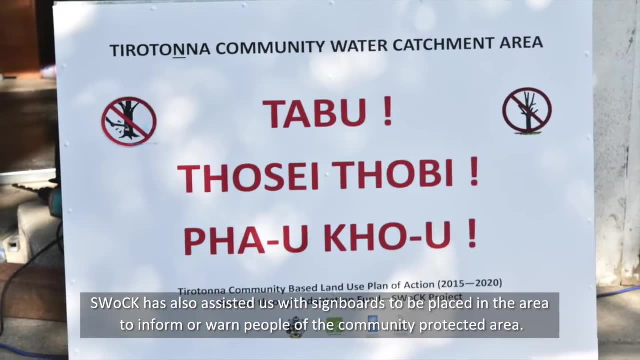 SHOC is also helping Mifala to provide them with sign boards for Mifala to put them up in that area So that if anyone comes past or comes to look at them, this one has a protected area for Mifala. 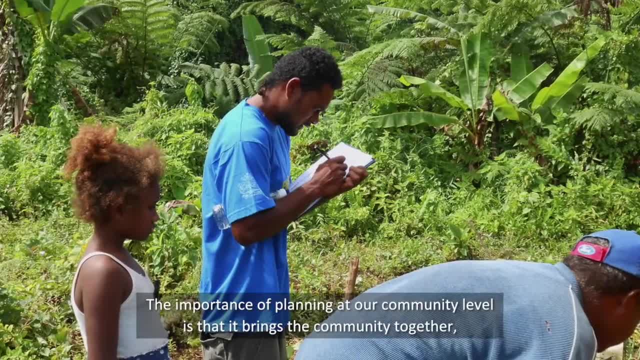 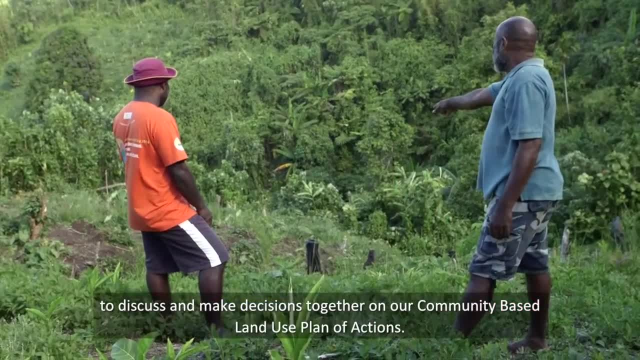 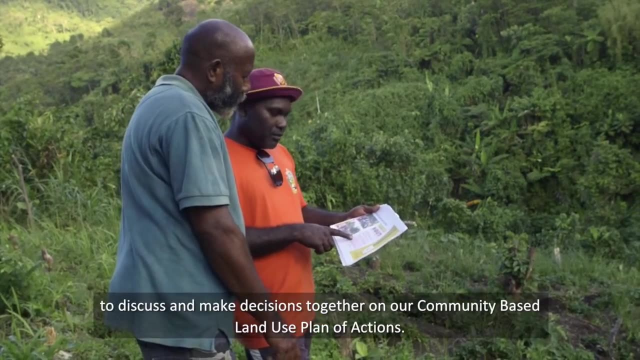 The important planning of the community for Mifala now is bringing Mifala community together for Mifala to sit down and discuss and make decisions on the Mifala community-based land use plan of action for Mifala With the SHOC support. 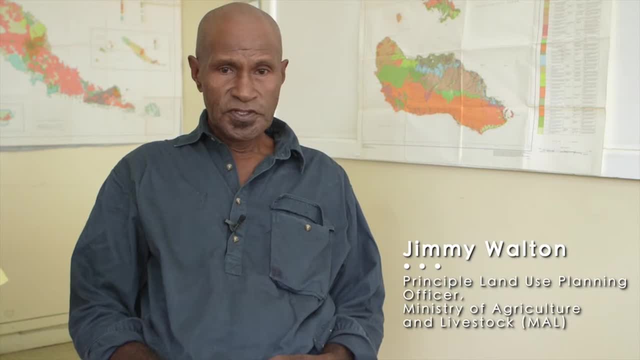 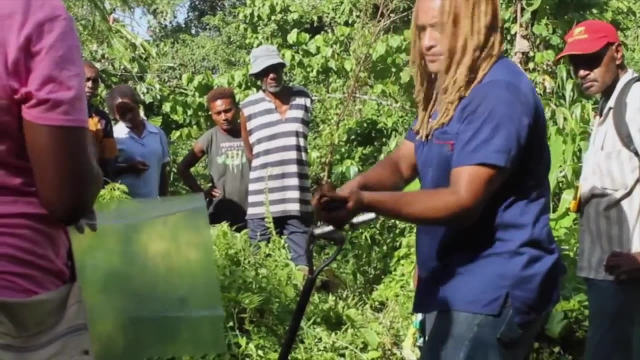 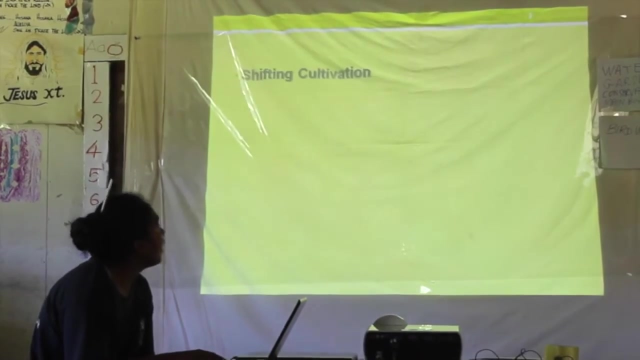 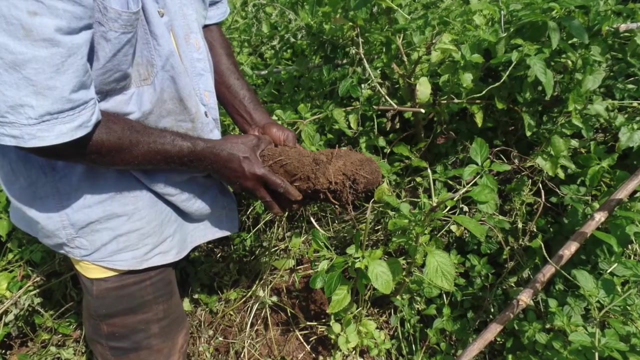 the ministry has managed to go down to the communities and teaching them about the different soil systems they have, the different land systems in terms of crop suitability, which crops are suitable for the different types of land they have, and also in good soil management practices. 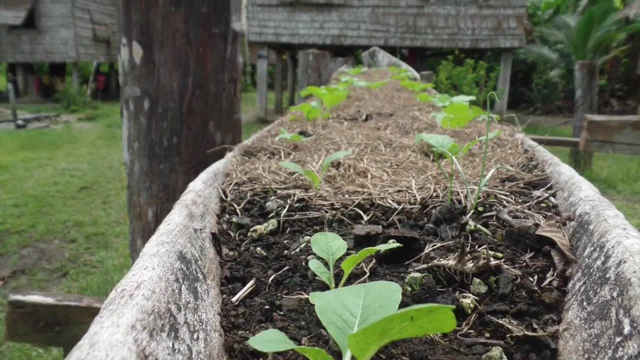 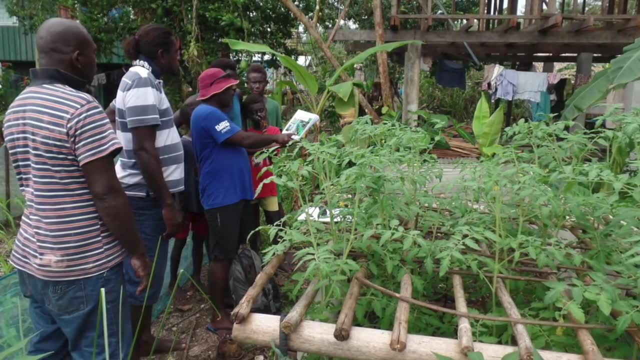 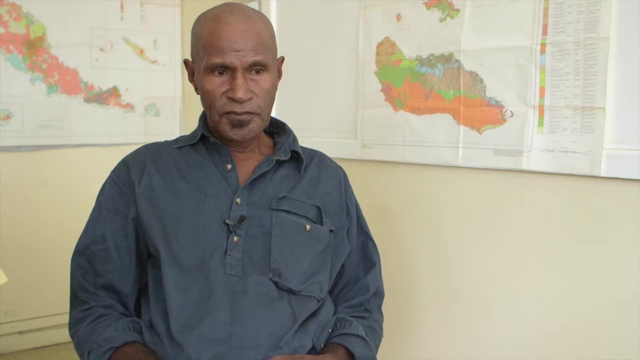 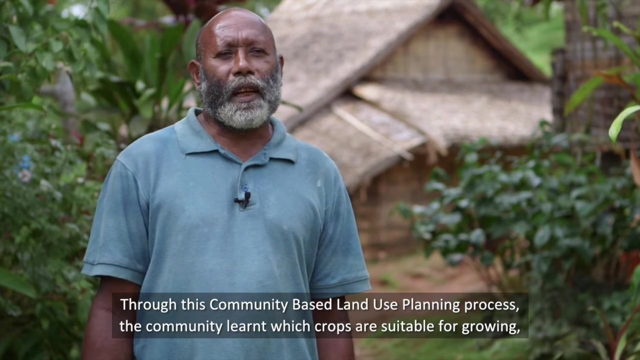 so that they can be able to understand the limitations of their different soils and, in good soil management practices, how they could improve on their soils for continuation of food production. So through this Mifala community-based land use plan, Mifala community just realized. 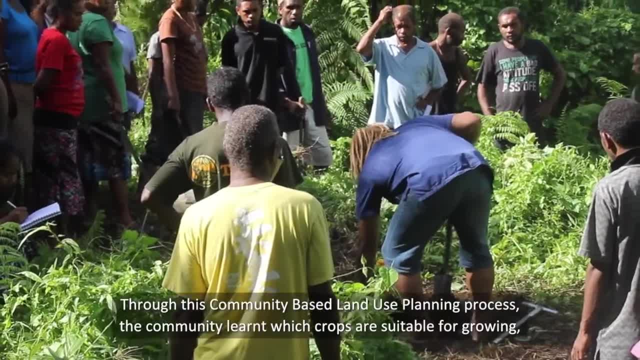 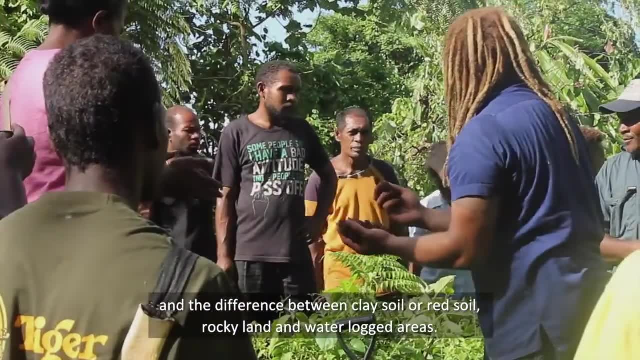 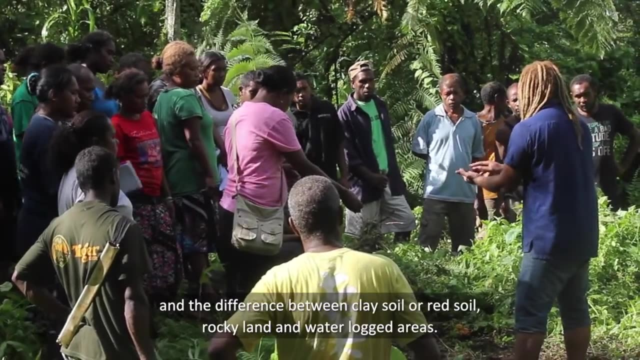 which crops are suitable for growing on land where there is clay or red soil and which crops are suitable for growing on land where there is soil and rocky soil and other soils where there are waterlogged areas. I want to tell Mifala people. 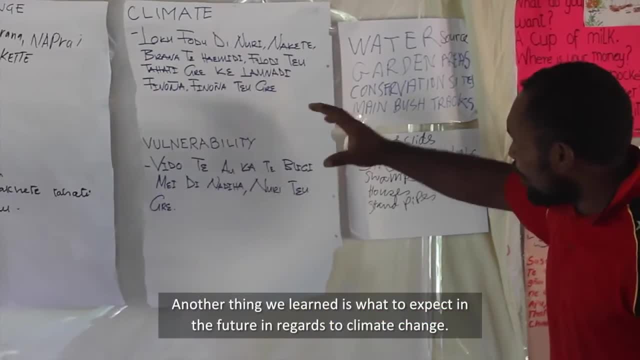 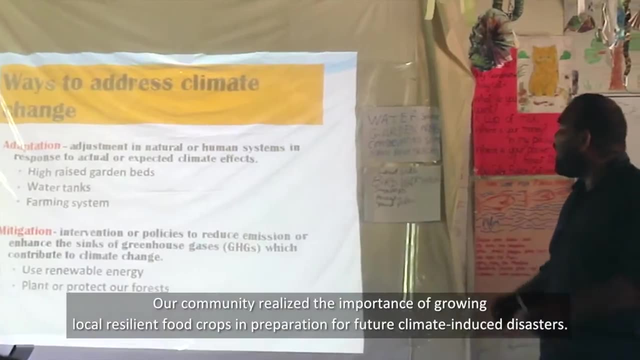 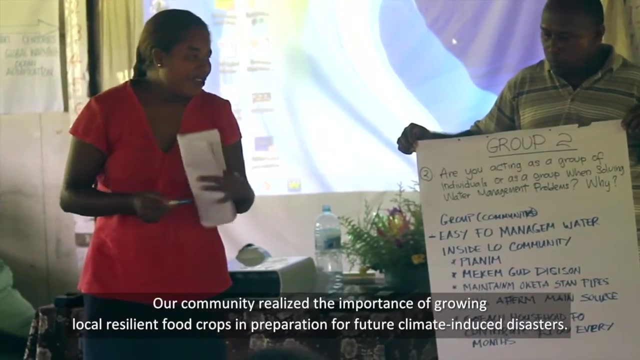 how they should look forward to the different climate changes that are happening. today. The community just said that the different types of food are good for the future and for the future and if anything happens to the environment or the climate or the kind of food that is important for us. 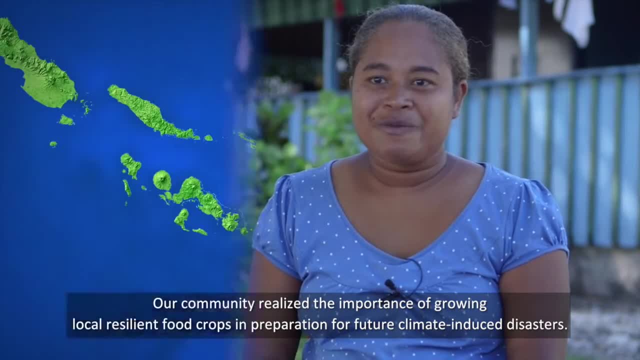 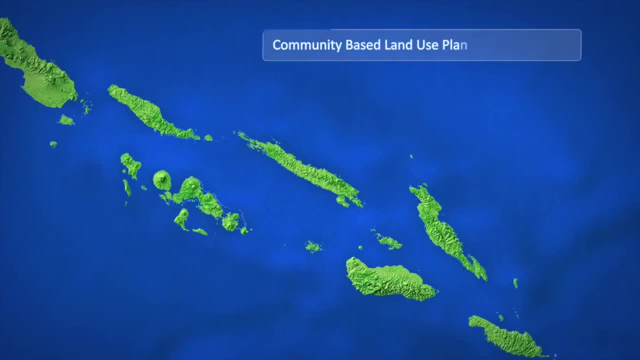 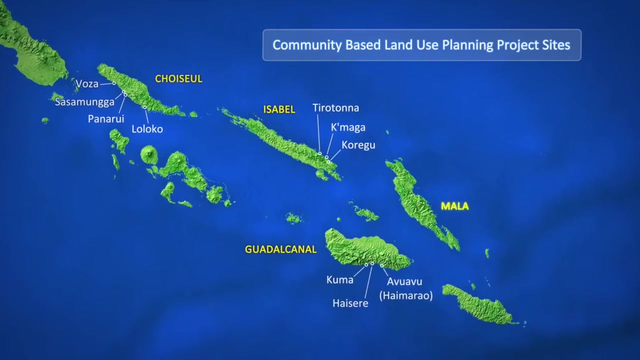 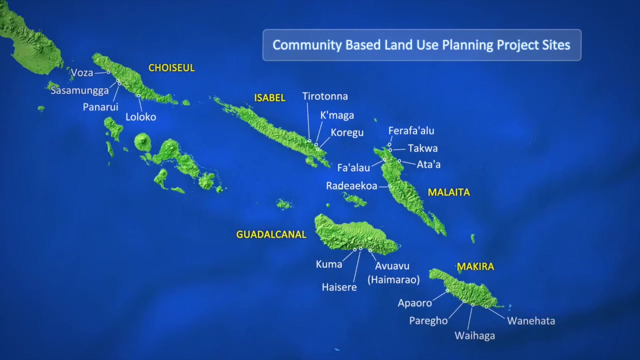 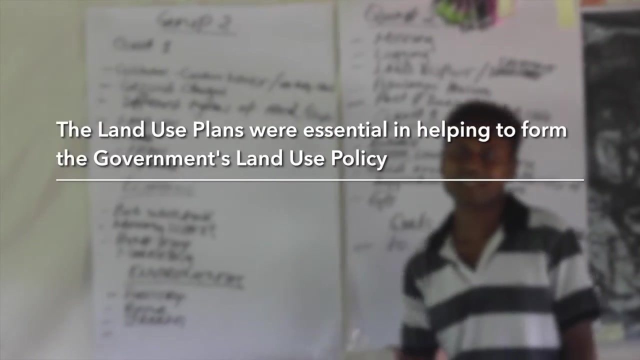 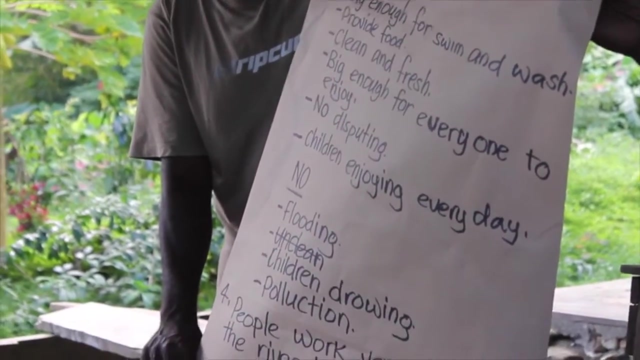 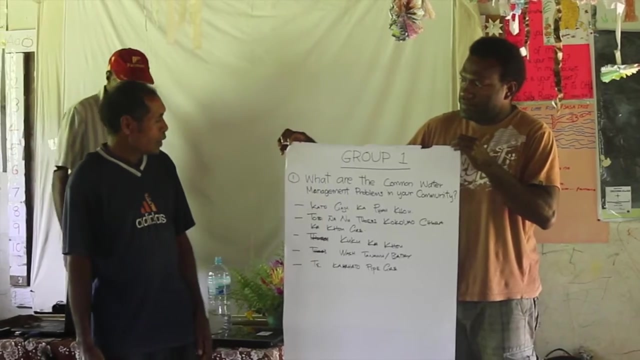 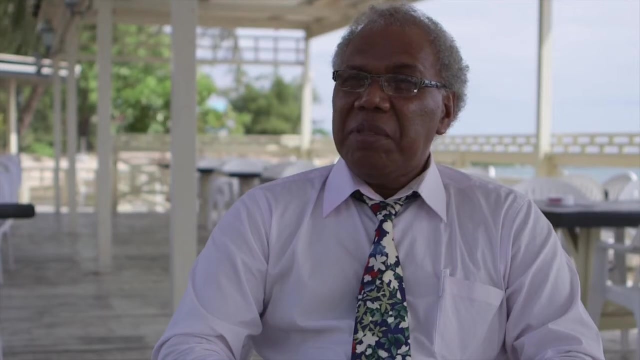 that is what Mifala is learning at the Mifala workshop. The쪽 project has assisted a lot in the development of the land use policy. The project has funded the technical assistance, assistance required to to begin the formulation and that has taken some time, which. 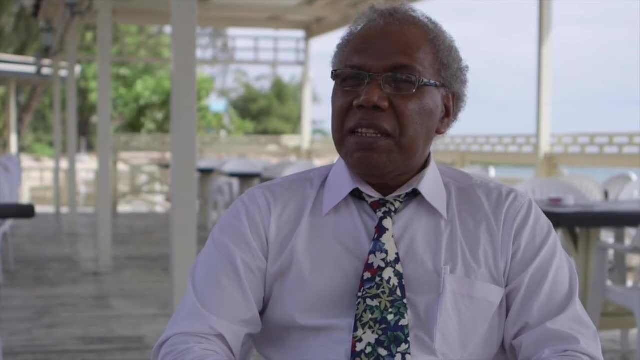 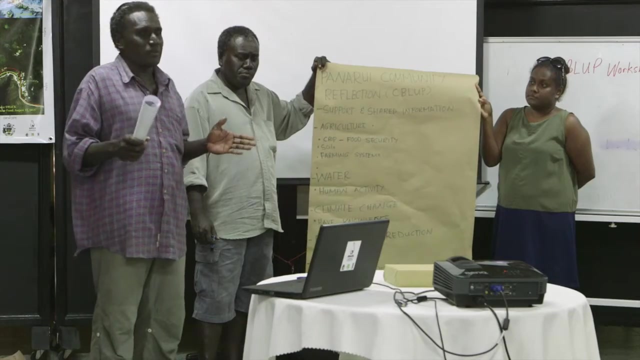 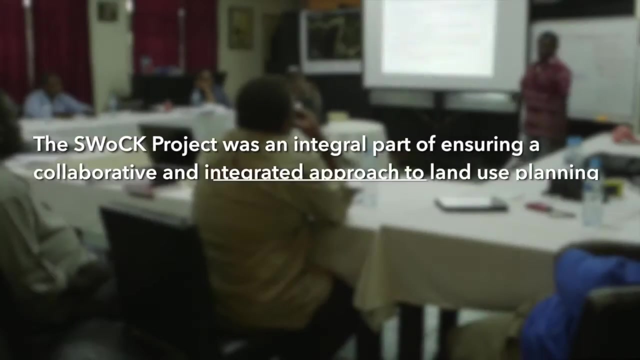 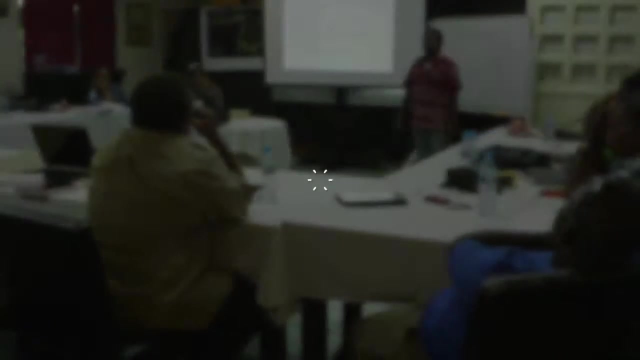 fortunately we have come to the end of that process. i think the policy is now ready to be endorsed by cabinet, sometimes soon. so i think the the project itself has assisted quite a lot towards the issue of land use planning and land use policy as a whole. this fellow integrated approach here. 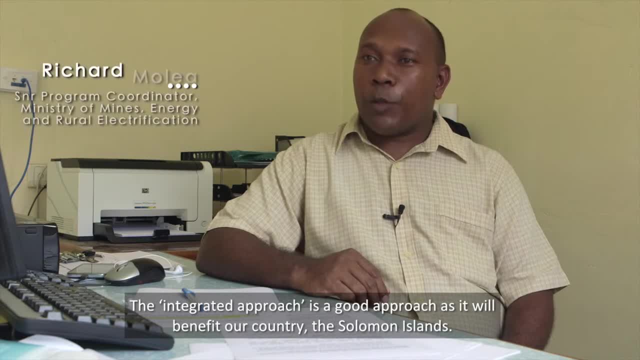 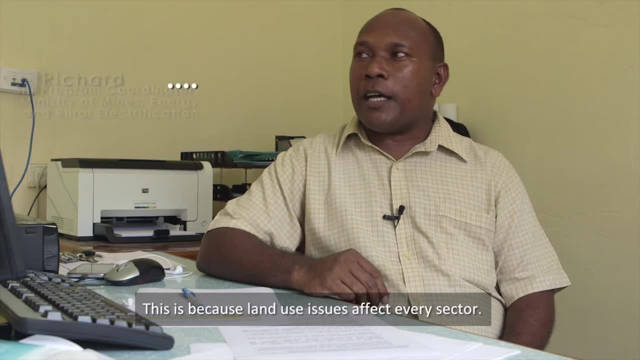 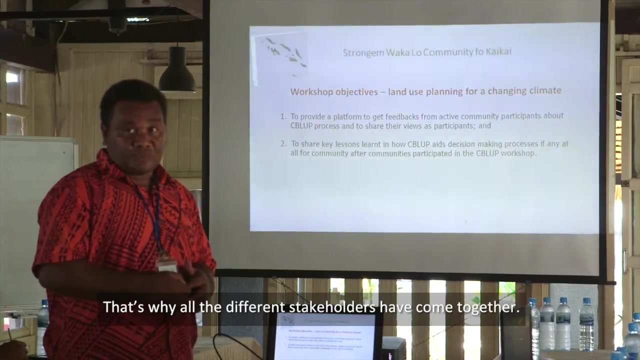 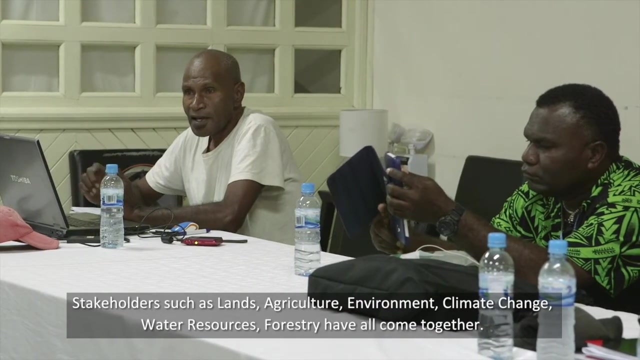 have me good one and him by benefiting someone- island, because all this land use are running some issues here. have me something affecting every sector. okay, every sector as the wire now, by looking this one: okay, hand me where me for everyone. come together all different stakeholders: lands, agriculture, environment- okay, climate change, water resources, forestry. 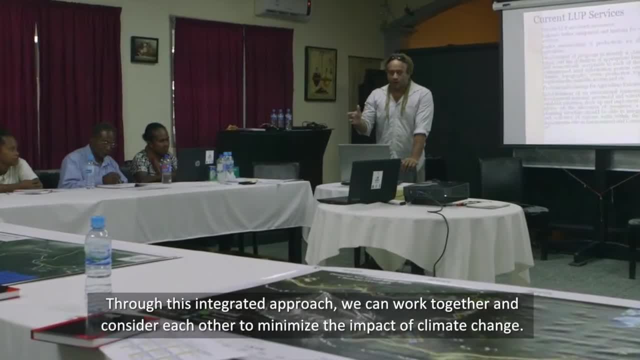 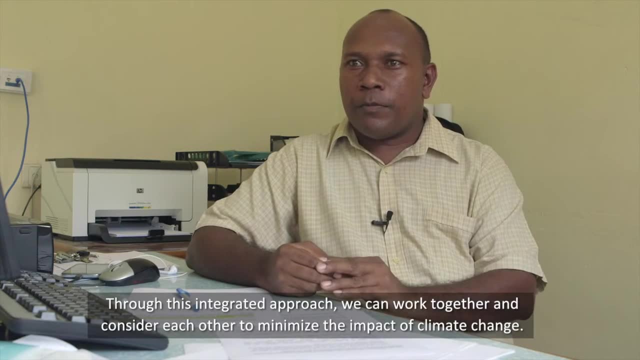 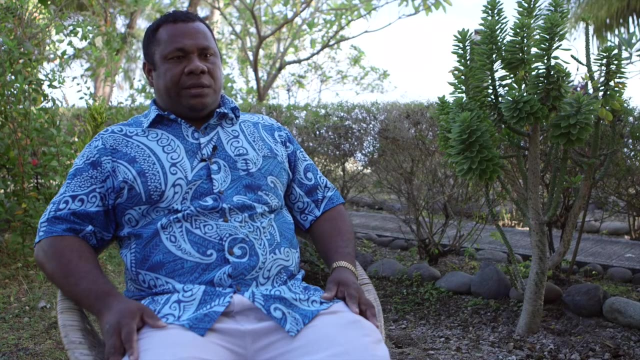 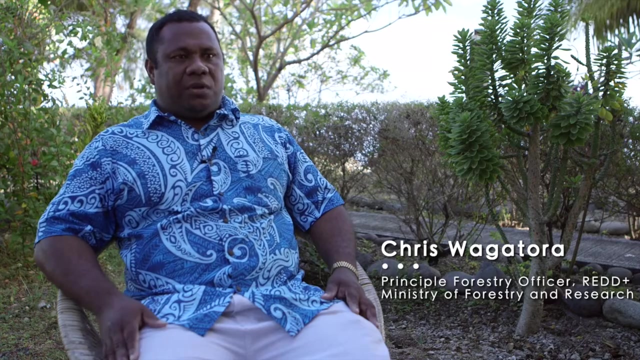 everyone come together and by coming together- me for survey, work together okay. consider each other. try lock, minimize him. okay. impact block climate change. the climate change issue is a cross-cutting issue which affects all the sectors in many ways and in different forms, so this new collaborative approach or integrated approach will help a lot of our communities. 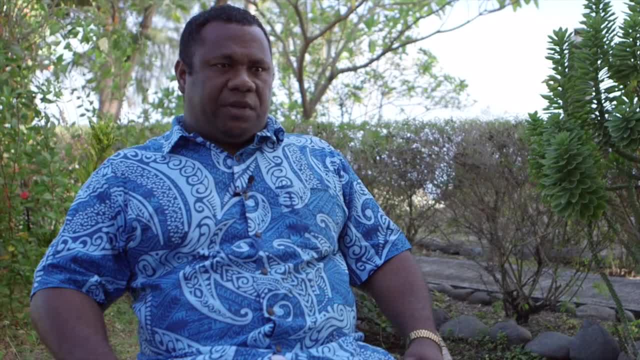 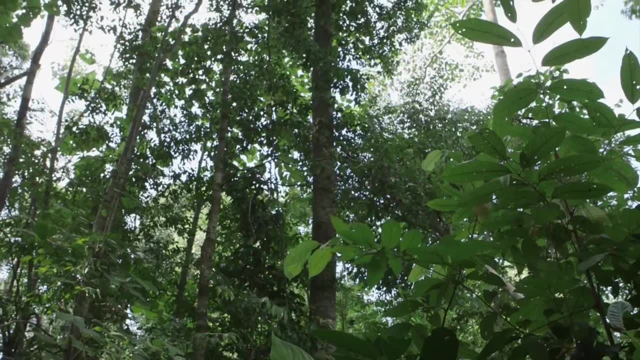 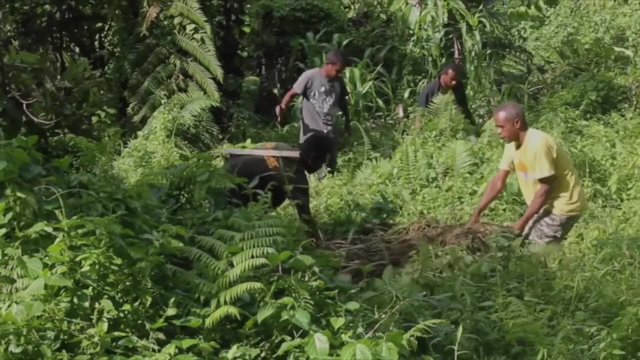 a swap project really helps me a lot in my work, since there are many projects. There are three phases of REDD+. The first phase is the initial phase, which is through capacity building and awareness. So SWAC really helps me a lot to be part of the team who do the awareness at the local. 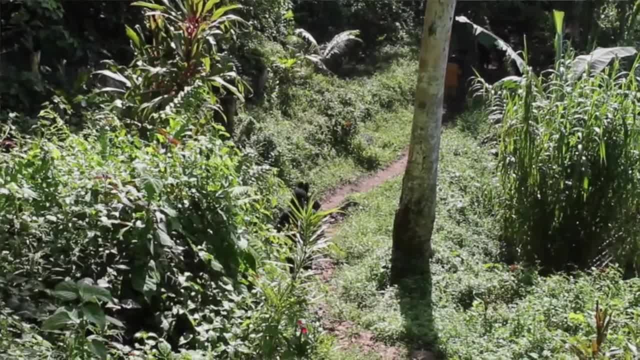 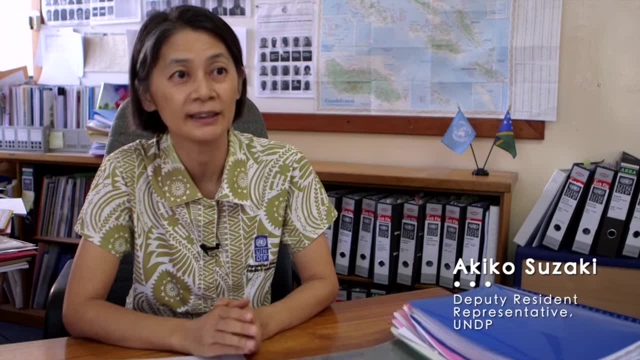 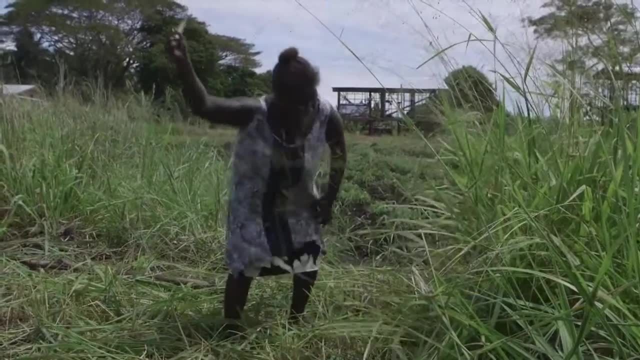 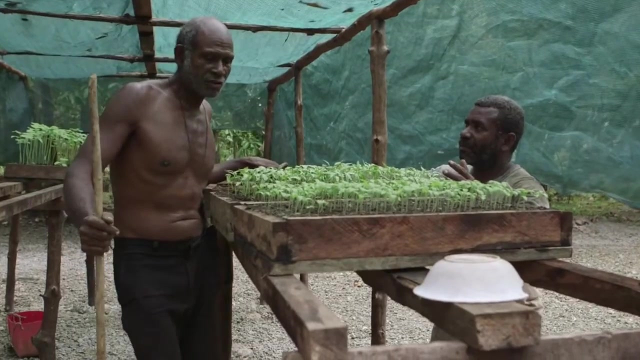 communities. So it really helps me a lot in the REDD+ initiative awareness to the local communities. The SWAC project has been making contributions in increasing residents of people and food security in rural and very remote communities. In this given climate change situation, the SWAC project has been empowering the people. 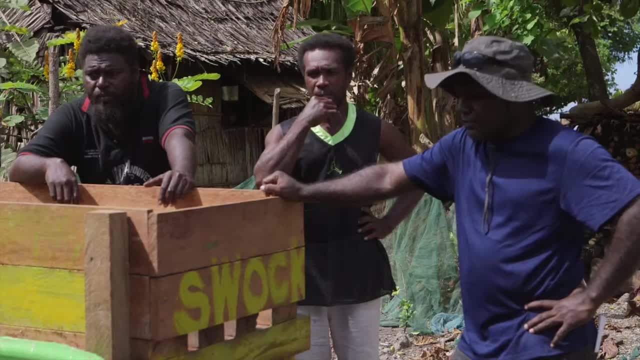 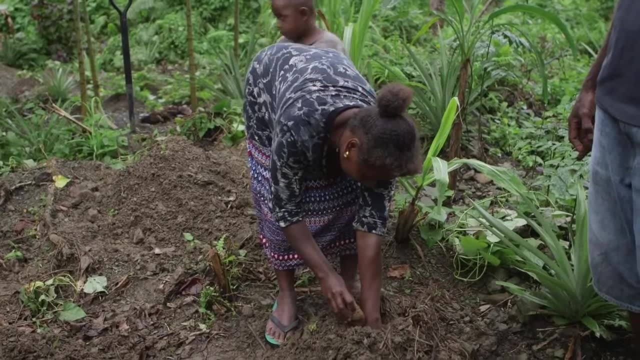 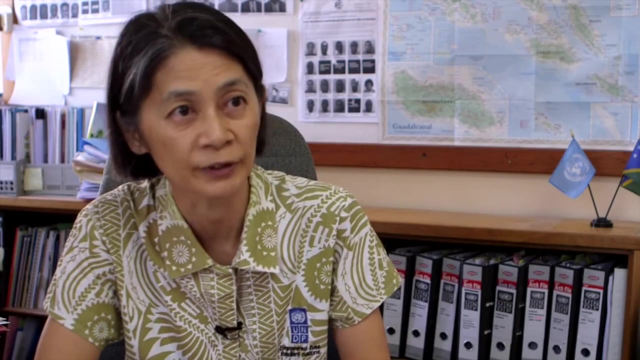 in rural and most vulnerable areas in making their decision, in planning and implementing their own food security plans. This is where UNDP makes a difference in helping the most vulnerable communities in Southern Islands In this given climate change situation. 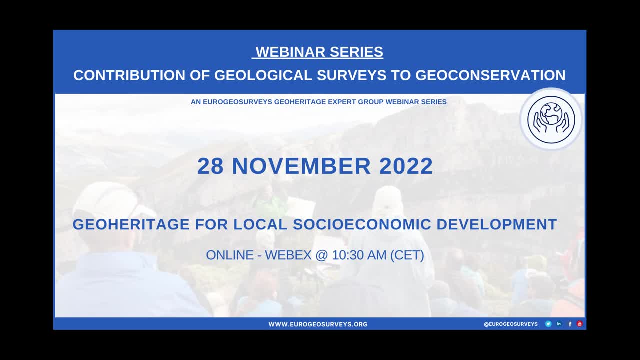 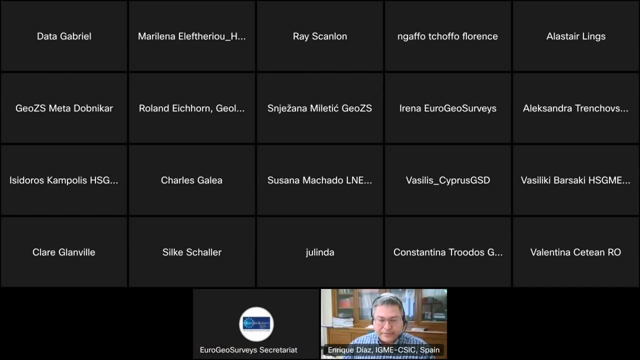 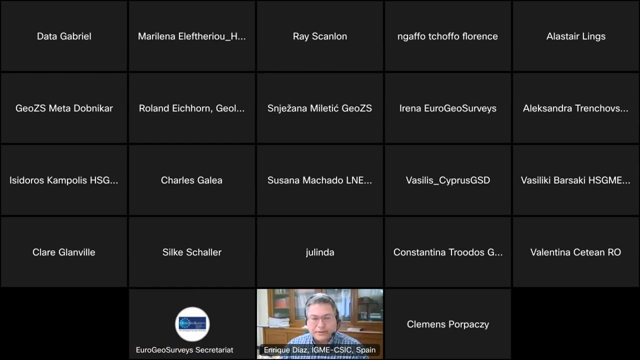 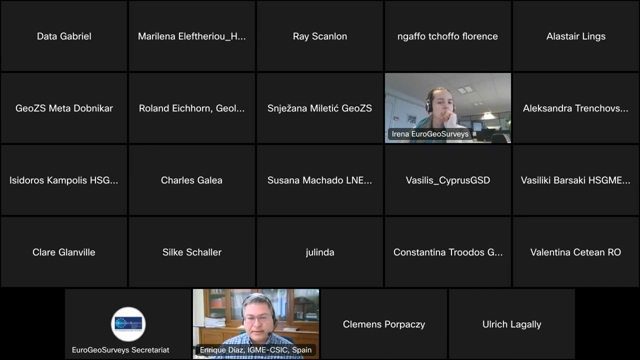 Thank you all for coming today to this first session that we are having organized thanks to the Eurogeoservice Secretariat and it was thought from the GeoHeritage expert group to have several sessions related with GeoHeritage in different aspects. The session for today: 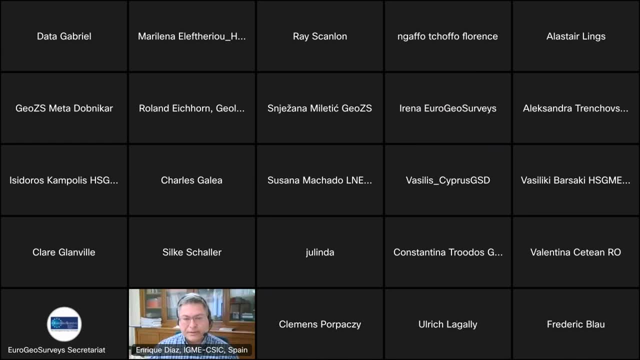 the first one of the GeoHeritage expert group is called GeoHeritage for local socio-economic development, And we are going to have three keynote speakers. The first one will be Dr Roland Eichhorn from the Bavarian Geological Survey. We will be talking about a bottom-up. 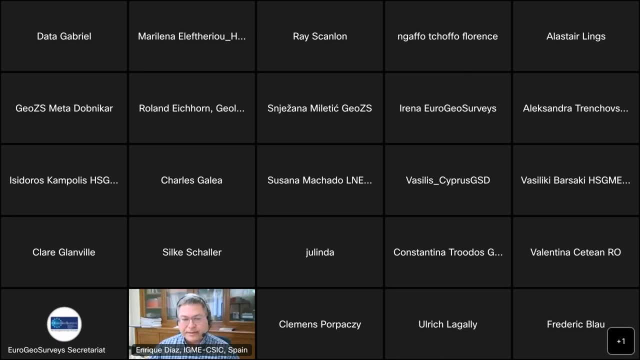 approach to enhance visibility. Then we will also have Claire Glanville, from the Geological Survey of Ireland, who will be speaking about county-level audits in Ireland to promoting and protecting local GeoHeritage. And finally we will have Nicolas Charles from the French Geological Survey, the BRGM, who 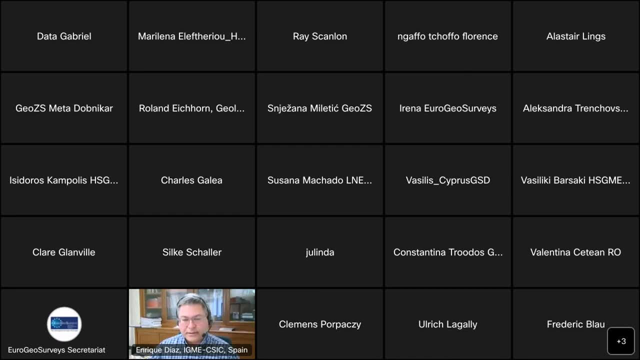 will be speaking about highlighting GeoHeritage in the world's leading tourist country. Nicolas Charles is a member of the European Geo-Geographic Survey. He was the chief executive officer of the European Geo-Geographic Survey. Then he visited for two weeks with the European 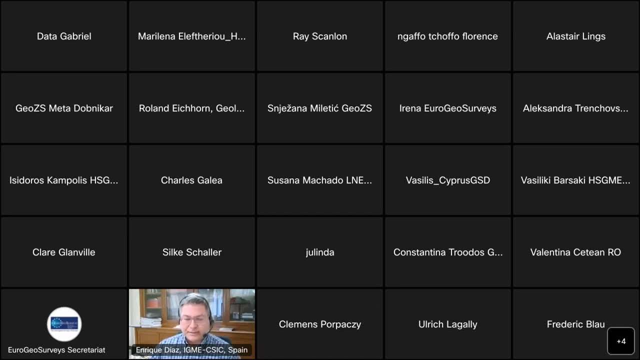 Geo-Geographic Survey in time. You are welcome to speak to him and we will ask him about which countries are some of the most important sources of knowledge in Geo-Geography and culture. May I say the first two speakers of the evening. Marc told us that about the European.